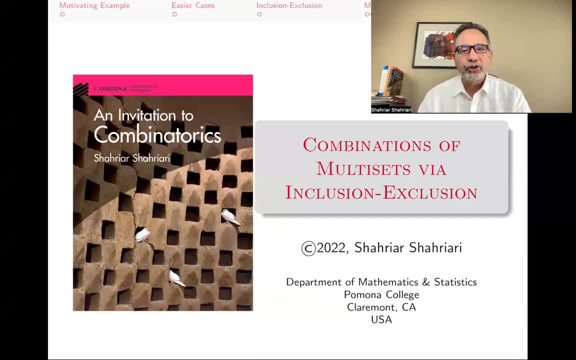 Hello, my name is Shahyar Shahyari and this is a lecture in a series of lectures on introductory undergraduate combinatorics, based on my book An Invitation to Combinatorics. The subject of this lecture is combinations of multi-sets via the inclusion-exclusion principle. 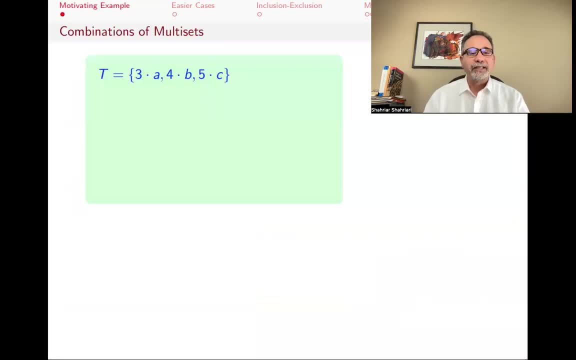 So let's get started with a motivating example. Here's a multi-set. A multi-set is a set, except its elements might be repeated. So this set T has three copies of A, four copies of B and five copies of C. It has three types of elements, but these numbers have repetition. 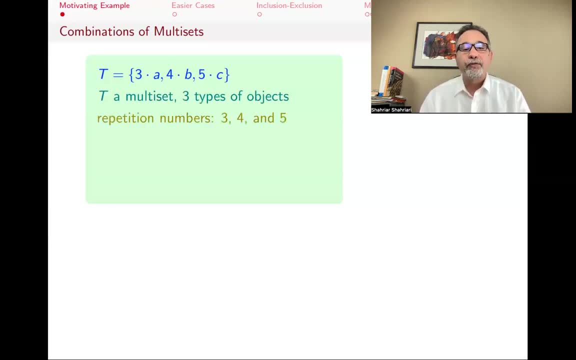 numbers or multiplicity: three, four and five. There are three copies of A. those copies of A are all identical- four copies of B- those are all identical- and five copies of C, which are also identical to each other. And what we want to know, for example, is how many. 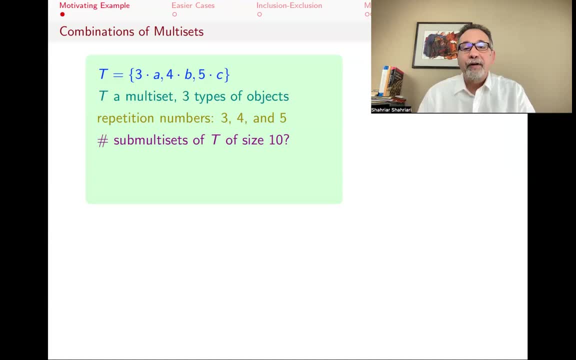 of these elements are repeated. So let's say that we have three copies of A, four copies of B. sub-multi-sets can be find of this set T of size 10.. So I want to pick 10 elements. I want to know. 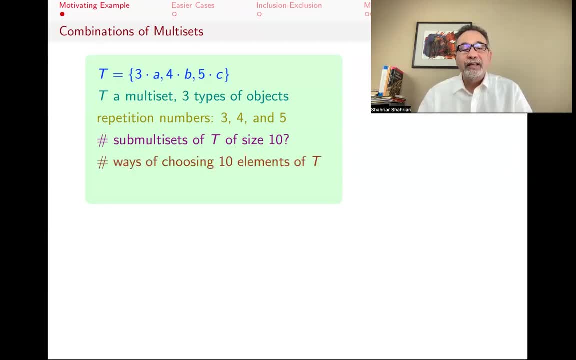 how many different ways I can do that. Another way I could say the same thing is that I want to choose 10 elements of T. However, elements of T are not all different from each other. Some of them are the same as each other. Another vocabulary one uses for these is the number of. 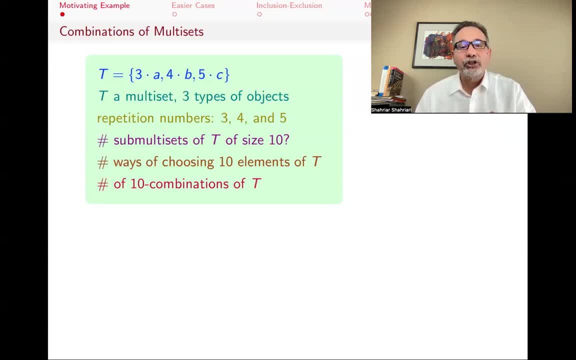 10 combinations of T. The problem with saying 10 combinations is that you don't quite know whether or not you're talking about a multi-set or a set. Sub-multi-sets makes that a little bit more clear, but all of these would be the same thing. We can translate this question to different. 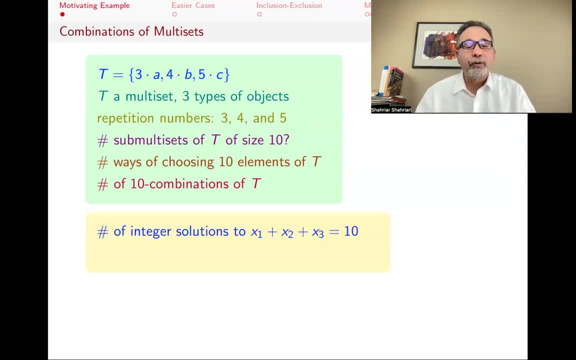 kinds of questions in combinatorics. We like to do that. So, for example, one way to recast this problem, look at it from a slightly different lens, is to say that I want the number of integer solutions, solutions that are integers to the equation x1 plus x2 plus x3 equals 10,. 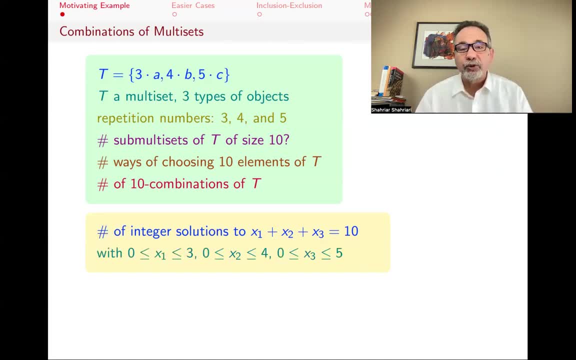 with the conditions that x1 is greater or equal to zero and less than or equal to 3, x2 is between zero and 4, and x3 is between zero and 5.. x1 is going to be the number of a's that I pick, x2 the number of b's and x3 the number of c's. And as soon as I have a solution, 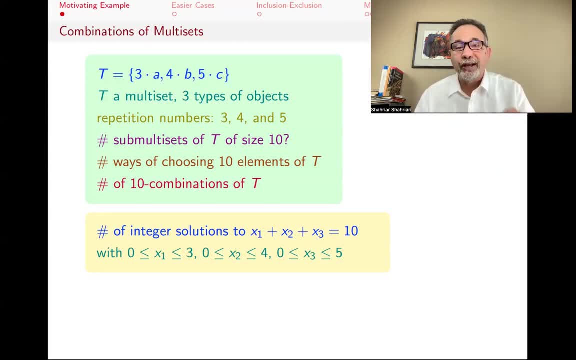 to this equation an integer solution. integer solutions for x1,, x2, and x3, satisfying the conditions. I've told you how to pick the 10 elements of that sub-multi-sets And vice versa. if you tell me how you want those elements to be picked, you are giving me a solution to this. 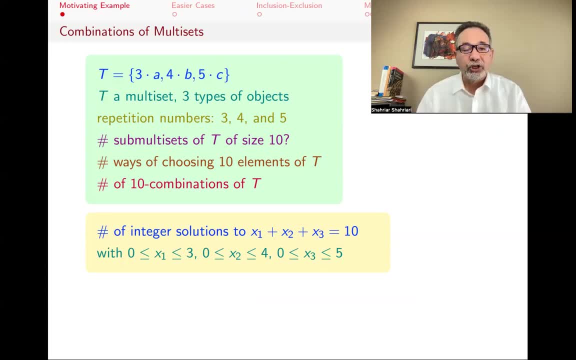 equation x1 plus x2 plus x3 equals 10, with those conditions. So this would be another way of recasting the question. We have seen many in previous videos. in other videos we have seen many combinatorial questions that like to be cast in terms of the number of integer solutions. 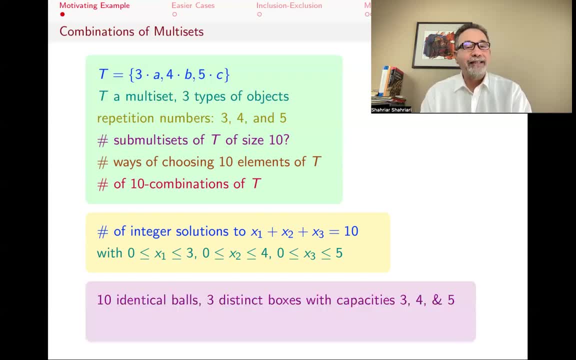 and number of integer solutions. We can also cast this or look at this from the lens of balls and boxes. So you can say that we have 10 identical balls and three distinct boxes, but these boxes have capacities. The capacities of these boxes are 10 identical balls and 3 distinct boxes. 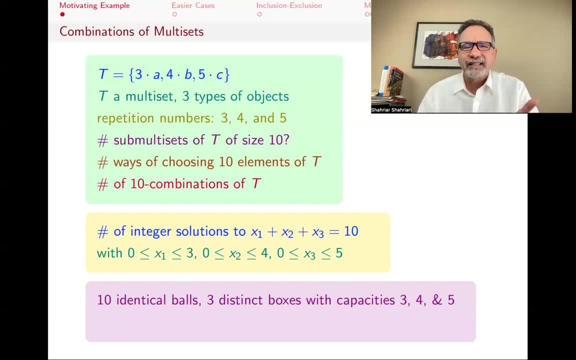 or 3,, 4, and 5.. In fact I didn't have to say distinct boxes because since their capacity is different, they are sort of distinct, But three distinct boxes with those, and I want to know how many ways I can place the 10 balls into these boxes, making sure that the first box doesn't 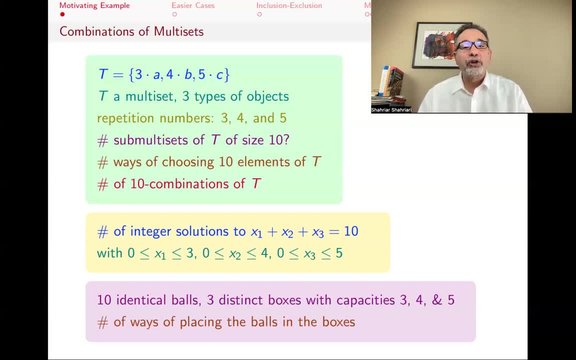 get more than 3,, the second box doesn't get more than 4, and the third box doesn't get more than 5.. So if you put a ball in the second box, then that means that you're picking one of the second. 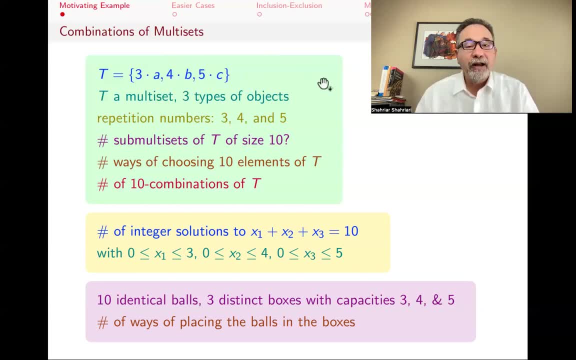 elements, one of the b's, And because the capacity is different, you can put a ball in the second box and the capacity of that box is 4, you're not never going to say pick more than 4.. And you have 10 balls, and that's what you want. You want to choose 10 things. Those 10 balls are telling you. 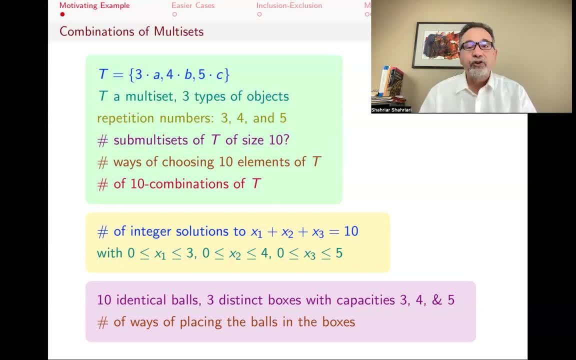 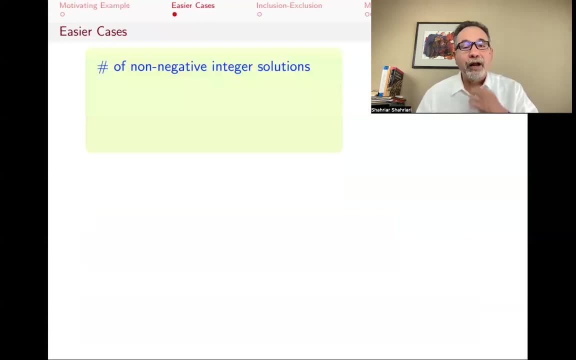 who to choose. Evidently, these are different versions of exactly the same problem, and that's what we want to solve in this video. So, first of all, there's some cases of this problem. I mean similar kinds of problems, sub-multisets of a multiset that we have already done So for. 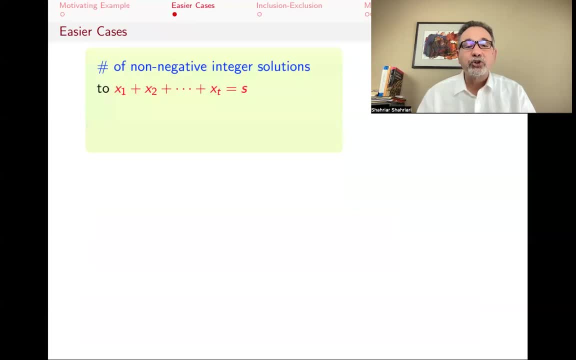 example, if someone has asked you the number of non-negative solutions to x1 plus x2 plus x2 equals s, with not any conditions on it, which is the same as saying: find the number of s combinations of this multiset, but here the multiset, the multiplicity numbers, or 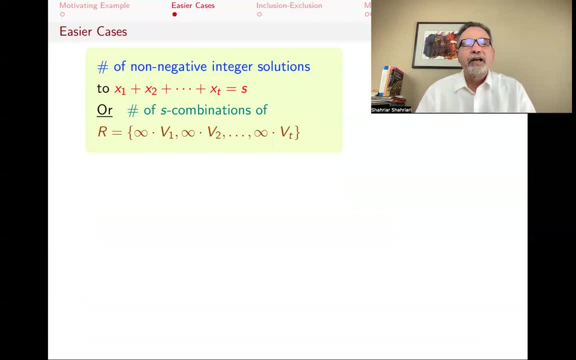 the repetition numbers are infinite. They don't actually have to be infinite, It's just that they have to be more than s or s or more, in the sense that when you're picking things, you're never going to run out of one of the elements In that case- we have seen that in other videos- that you 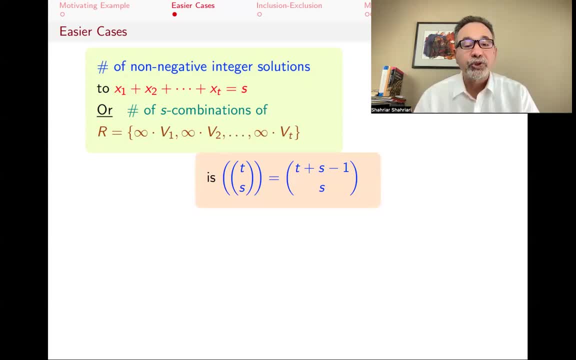 should look at that. the answer is t multi-choose s, and t multi-choose s is given by t plus s minus one choose s. So this is a subject of other videos. Go watch those. if you haven't seen those, You do. 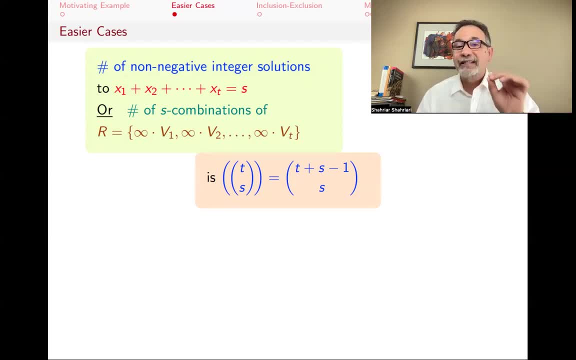 need to watch those and understand how to solve this simpler problem before we can answer a question about multisets, where there is restrictions on how many elements of each type we have. So if you don't have any restrictions, you can pick as many of them as you want. Type one element, as you want type two elements we want. We have done this. 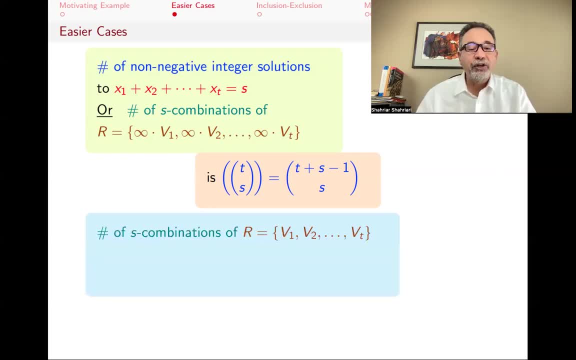 previously and the answer is t, multi-choose s. Another set time when we have done this is when we have: multiplicity numbers equals one, repetition numbers equals one, So number of s combinations of a set. or I just have one copy of v1, one copy of v2, and one copy of v3. That's the same as saying: 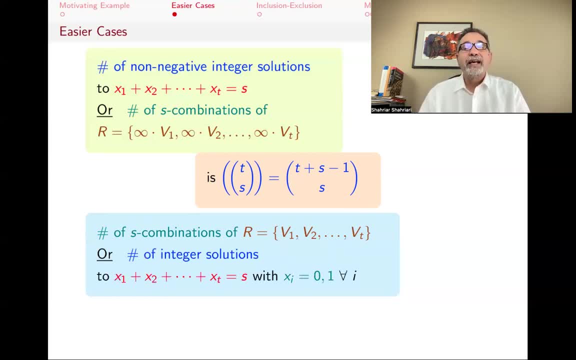 I want the number of integer solutions to x1 plus x2 plus xc equals s, but xs equals s, xc equals s, but I want each one of xs equals s and I want each one of xs equals s and I want each one of xs equals s. 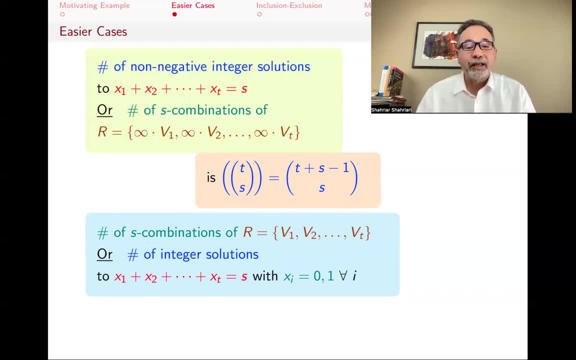 to be either zero or one. So I'm either picking them or not picking them, And this is clearly just going to be t choose s, because you have t objects and all you have to do is figure out which s you want to pick. So these two are special cases of what we want to discuss today, which is 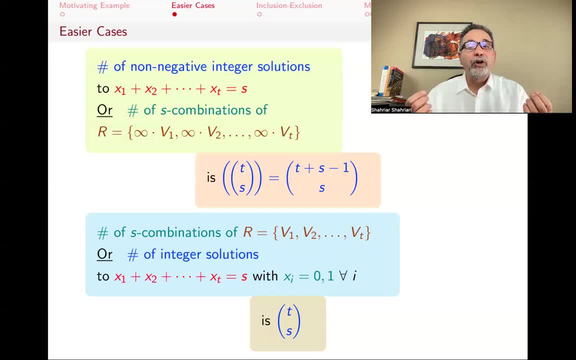 finding an s combination of a multiset where the restrictions aren't that the repetition numbers are all one or all very large, and they can be anything. Of course, this is going to be a more complicated situation and it will encompass the ones we have. 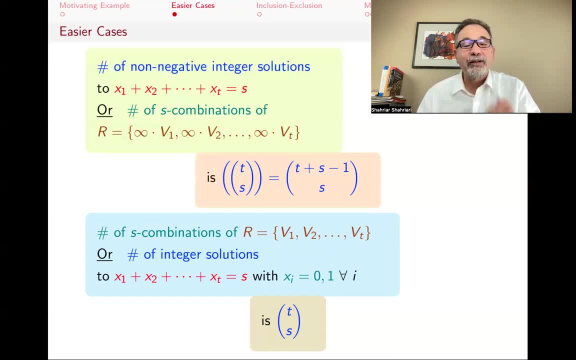 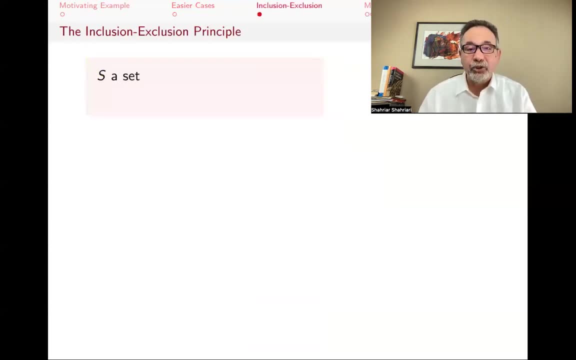 done before, and the answer is not going to be as nice as these. It's not going to be just a nice little formula that you can plug in. What we are going to do is we're going to use the inclusion-exclusion principle, and I want to remind you of that. Inclusion-exclusion is the 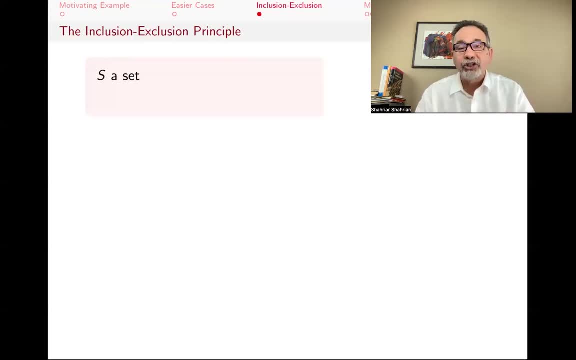 subject of another video that I would urge you to watch Again if you haven't watched that. that's the prerequisite for understanding this video. So if s is a set and you have a bunch of subsets of it, m subsets of it- a1,, a2, and am are subsets of s. 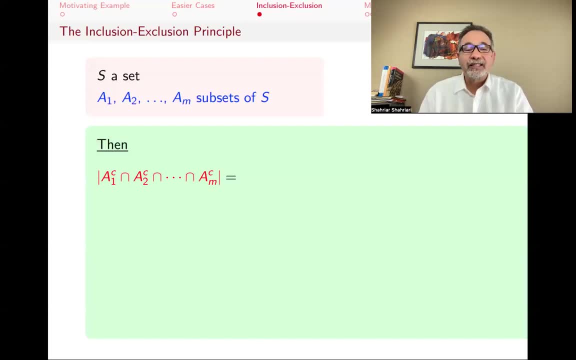 and you want to find the size of a1 complement intersection, a2 complement intersection am complement. Think of a1 as all those elements that have certain property and a2 another property and am a certain property and there might be overlaps in terms of those properties. Some. 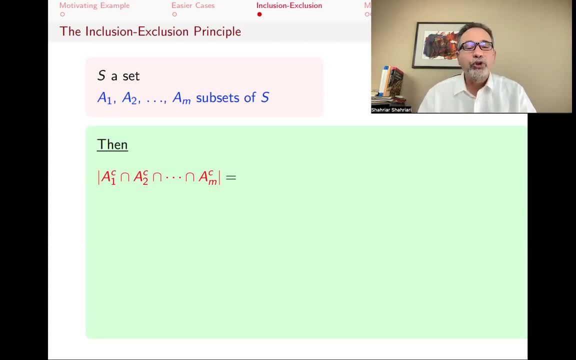 elements might have three or four of these properties or none of them, and what you want is the number of elements that have none of the properties. none are in none of these sets and the inclusion-exclusion principle tells us: well, start with s, that's everything, but that's too much. Then throw away all the things. 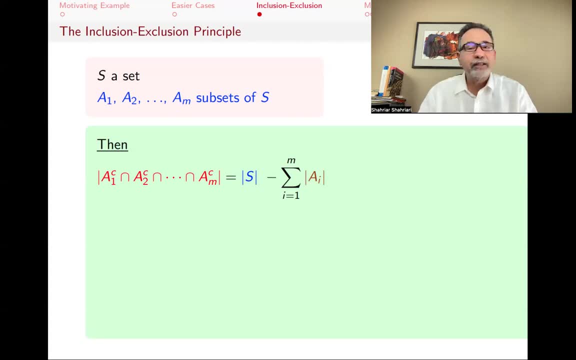 you don't want, which is the size of a1, the size of a2, the size of a3. Those are elements you don't want, but by so doing you have thrown out too much, because, for example, something that was: 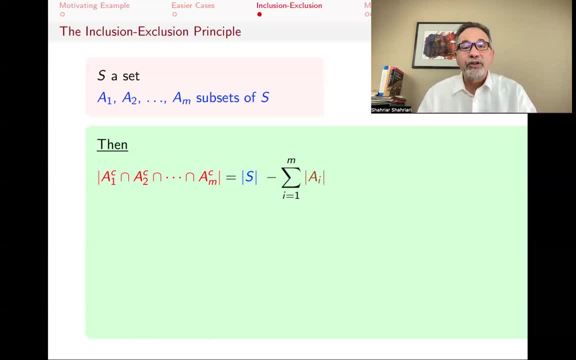 both in a1 and a2 was thrown out twice, whereas it should have been thrown out once, and so you need to put that back. We put all the intersections of two things back in, but now we have put it back in too much. 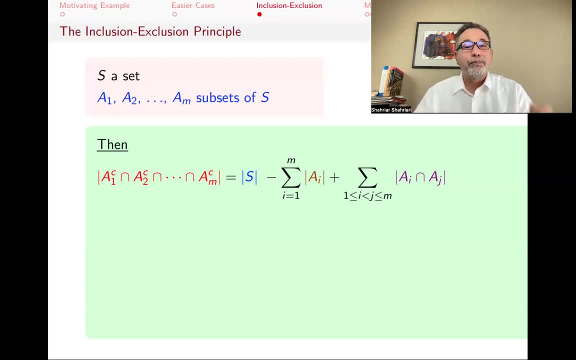 because if something was in three sets, then we have put back in three times, and we should not have done that, and so we have to take away all the intersections of three sets of distinct a's, the sizes of those intersections, and so on all the way till the end. Again, the proof of this. 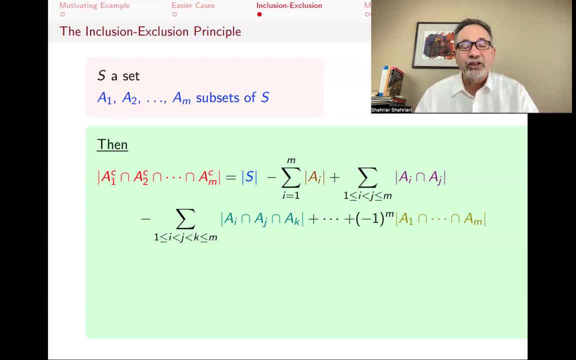 is in another video. We discussed that in some detail and give examples For this video. I'm assuming we know this, so just to make sure that we know what these summations are. the first sum is over all subsets of size 1 of 1 to m. so there's an element, there is a sum end here for each subset of size 1.. 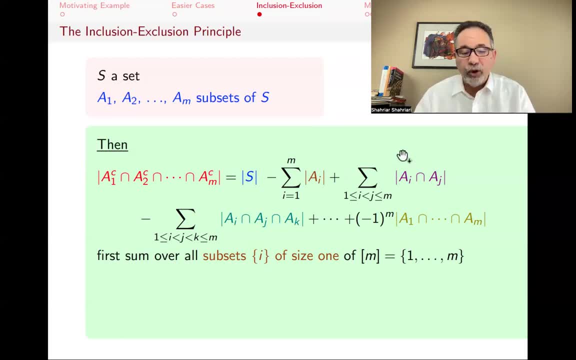 There's an a1,, a2,, a3, am, but for the second one there is one element, for there's one term for each subset of size 2 of m, and for the third one there is a term for each subset of size 3, and so on. so there's actually a lot of terms in this. 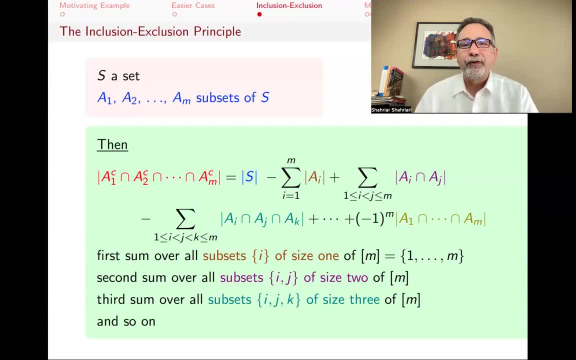 and this is why inclusion-exclusion is not usually one of the first places you go to solve a problem, because in general it can be quite messy and tedious, but sometimes you don't have any choice and sometimes it sheds light on things in ways that other methods do not. 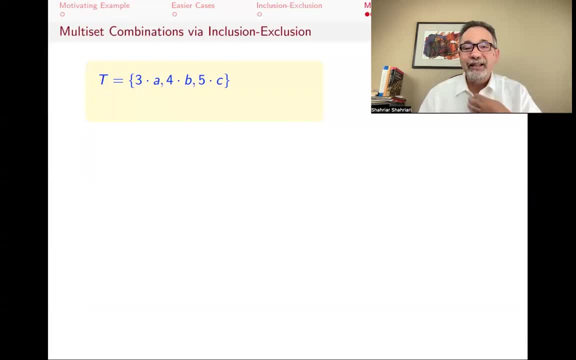 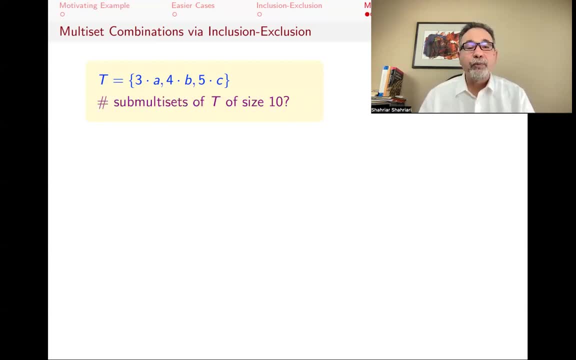 and repetition numbers 3,, 4, and 5, and what I want is the number of sub-multisets of t of size 10.. So what I will start with the setup is with inclusion-exclusion. you want to set up what? 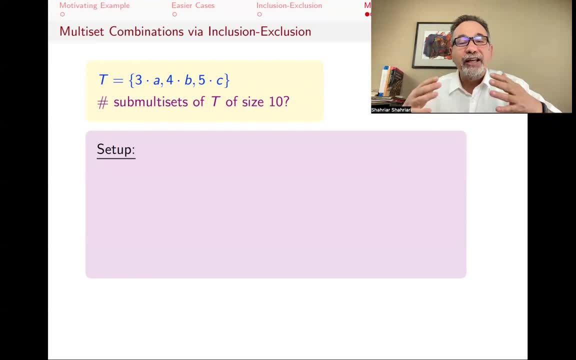 your ambient set, the s, the big set is. and then what are the sets? a1,, a2,, 2, am? and usually you set it up so that those are the sets of elements that you don't want and so that the thing you do want is the number of elements that are in either none of those. 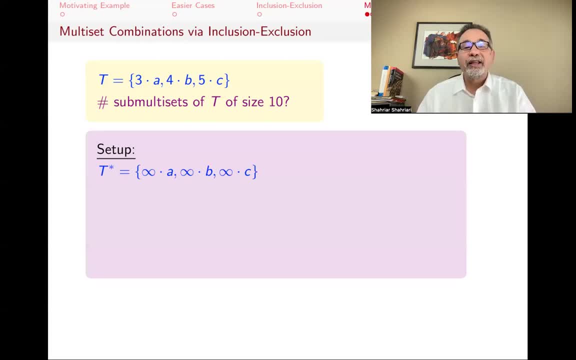 That's one way of setting it up. So setup here is that we start with a multi-set, that we know how to deal with a multi-set with infinite repetition numbers but the same type of elements. So we call that t star. T star has three types of elements but infinite number of each one of those and s. 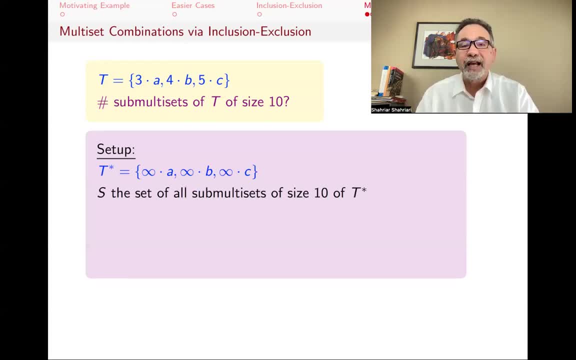 our ambient set is going to be the set of all sub-multisets of size 10 of t star. All the ones we want we're going to set up as a set of all sub-multisets of size 10 of t star. So we're going. 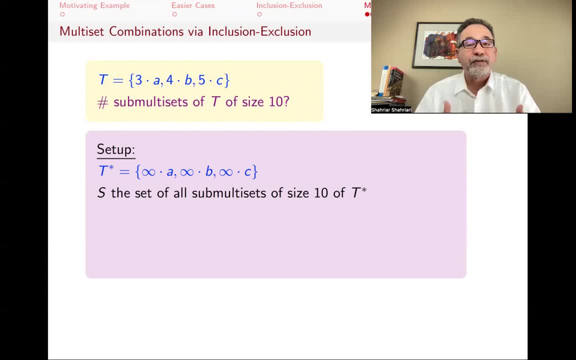 to set up as a set of all sub-multisets of size 10 of t star, All the ones we want, the ones of t. the sub-multisets of size 10 of t are among these. except some of these are the: 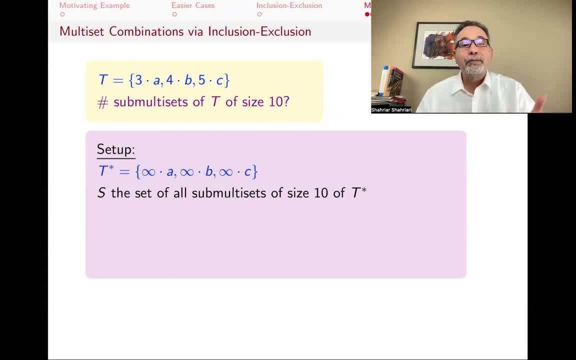 ones that we can't have because they're using too many a's, too many b's or too many c's. So we let a1 be sub-multisets of size 10 of t star with more than three a's, so four or more a's. 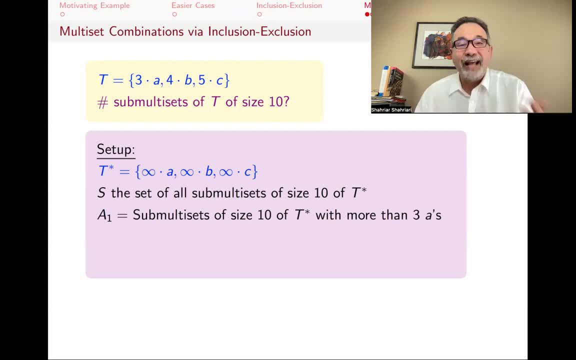 And again, that's a bunch of sub-multisets that I shouldn't be counting. if I count after I count the size s, and if I want to count the sub-multisets of t of size 10, I should not be counting elements of a1. Likewise, a2 is going to be. 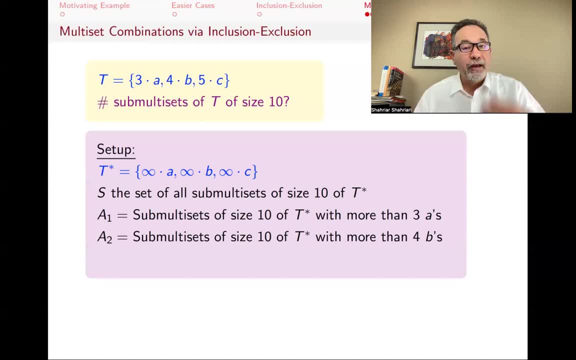 sub-multisets of size 10 of t star with more than four b's, five or more b's, And a3 is going to be sub-multisets of size 10 of t star with more than five c's. Again, a1, a2, and a3 are the bad. 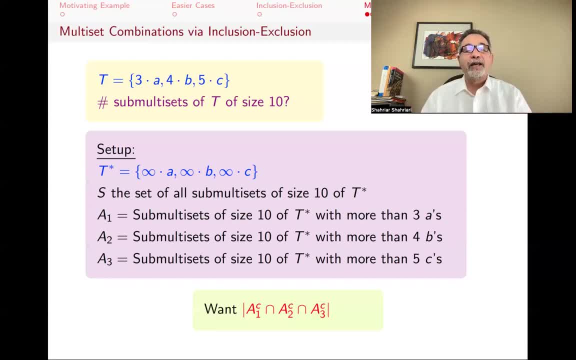 elements, the ones we don't want. So what do I want? I want the size of a1- complement intersection. a2 complement intersection, a3- complement, And now this is set up for us to use inclusion exclusion. I have an ambient set s. I have three subsets: a1,, a2, and a3,. 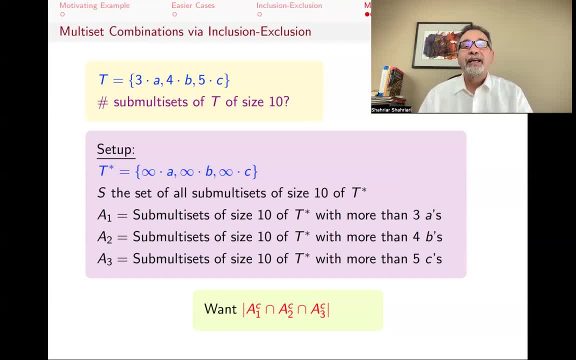 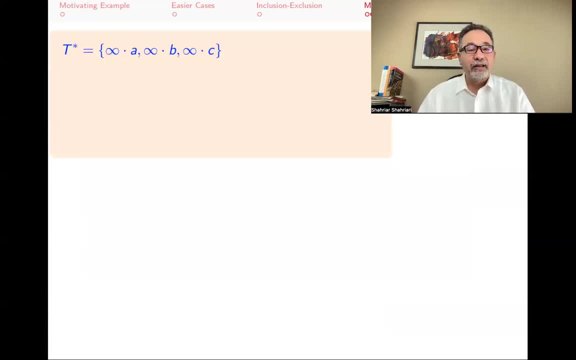 and I want the size of a1 complement intersection a2 complement intersection a3 complement. As soon as I have that, then I go and start doing it. So t star is again a sub-multiset with infinite repetition numbers and three types of elements, and s is the set of all sub-multisets of size 10. 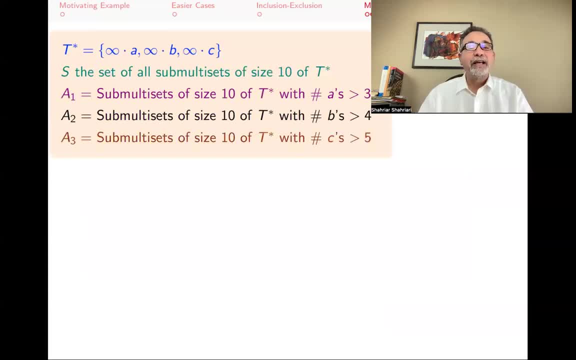 of t star, and a1,, a2, and a3 are as we set, And so now let's get our hands dirty and start working. So, to use the inclusion exclusion principle, I need the size of s, But the size of s is going to. 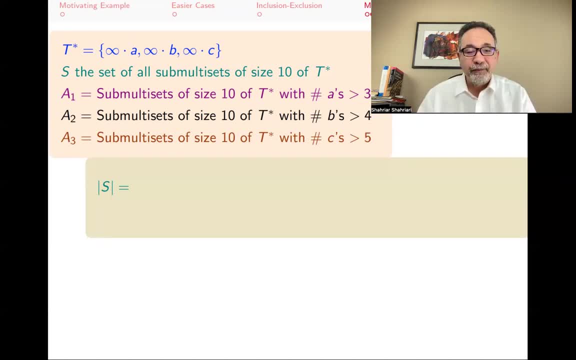 be. we already discussed that is going to be three multi-choose 10.. It's the number of integer solutions to. x1 plus x2 plus x3 equals 10, where there's no restriction other than x1 and x2 and x3. 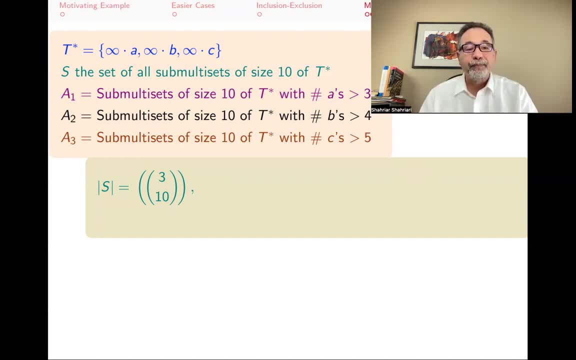 being non-negative integers, and that's a multi-choose number. Now, what about a1?? Well, a1, you want multi-sets of t star with more than three a's. That means you need at least four a's. Well, take the four a's and you know. 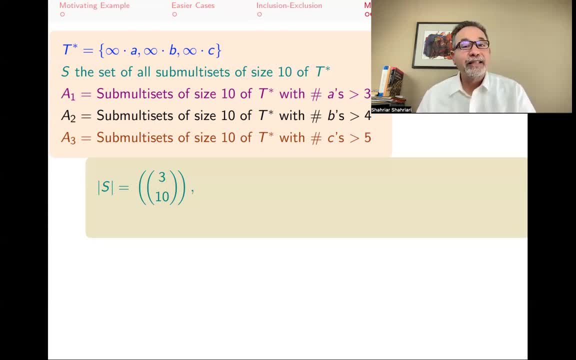 you need four a's, so take them, And then what you need to do is to make to pick six other elements of t star, And so you want the sub-multisets of size six of t star, again with no other restriction. 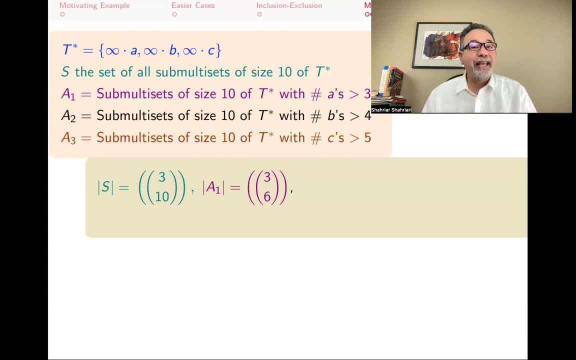 other than non-negative integer. number of them- And that again is the same kind of a problem- is three, multi-choose six. So you have three types of elements again in a sub-multiset, and you want to pick six of them, And so you want to pick six of them, And so you want to pick six. 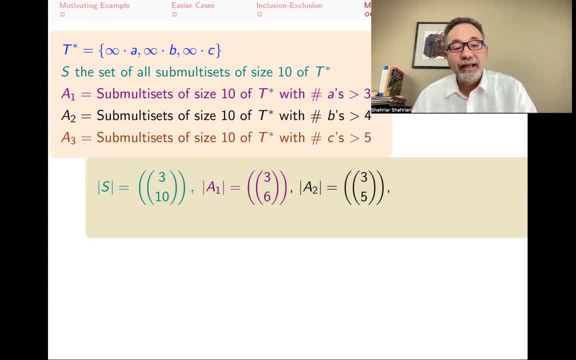 of them, And the same with a2.. A2 says that you want sub-multisets of t star with five or more. So give five or more b's. So give those five b's to your multi-set. And now, because you wanted, 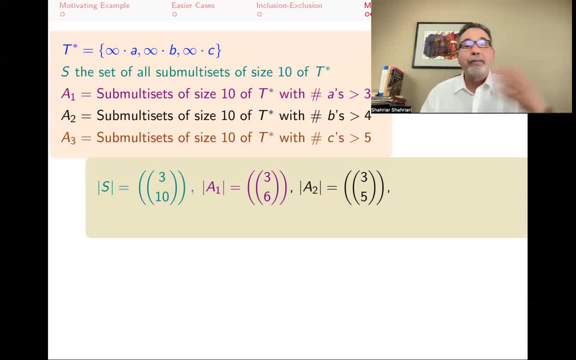 sub-multisets of size 10,. you have five more elements to pick from among the three types, But because there's infinite of them, there's no other restriction And the answer is going to be again: three, multi-choose, five. Again, watch the video on multi-set, combinations of multi-sets. 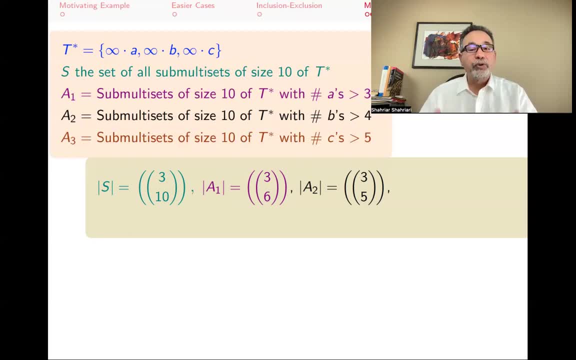 combinations of multi-sets And you'll see that there's no other restriction. And the answer is combinations with repetition, where we discuss this in general And a3 is going to be three multi-choose, four, again with the same thing, But we also need to find intersections. So what's the? 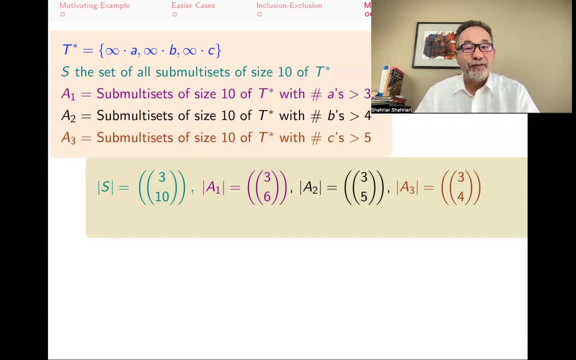 intersection of a1 and a2?? Well, that would mean that you want a sub-multisets of size 10, but you want at least four a's and at least five b's, because we want more than three a's and more than four b's. So that means four a's and five b's. And if you do that and if you give 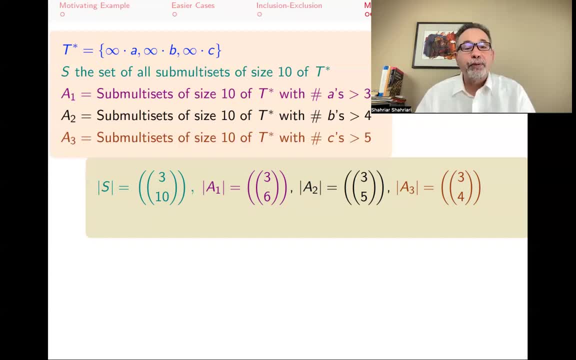 the four and the five. you're going to get a sub-multisets of size 10. And you're going to get a's and the b's, And then you just have to pick one thing, And that one thing could be a, b or c. 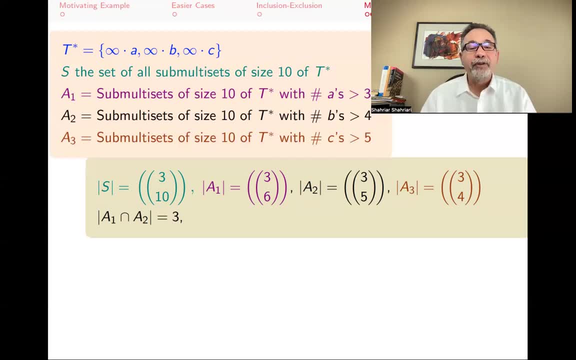 So a1 intersection a2 is actually just three. What about a1 intersection a3?? That means I need more than three a's, I need four a's or more, and I need six c's or more. Well, that's already 10.. 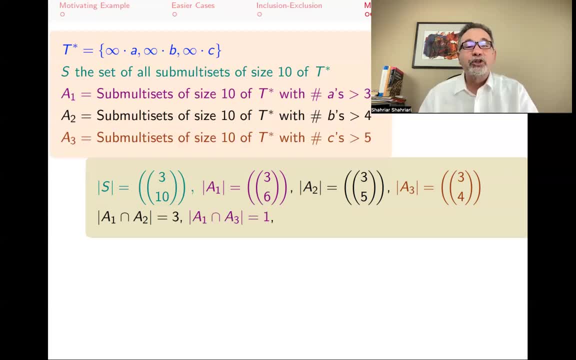 So I need to pick just four a's and six c's, and I don't have much choice. There's only one way to do that. So there's only one element in the intersection of a1 and a2. And that's the. 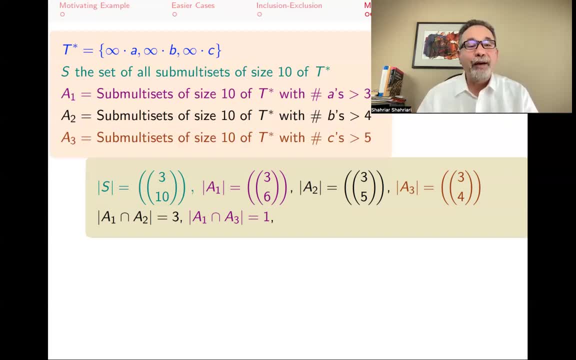 intersection a3 that has both properties of a1 and a3.. And what about a2 intersection a3 or the intersection of all three of them? That's zero. It's not possible to have a sub-multisets of size 10 of t star that has four a's, five b's and six c's. That's just too many. I can't have that. 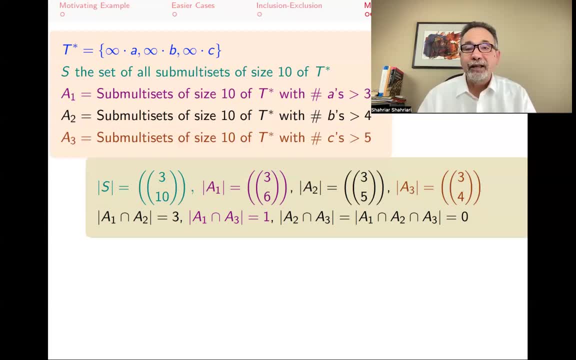 And so those are all zero. And so now I can apply my inclusion-exclusion principle And I can say write down the inclusion-exclusion principle in this case, which says that if you want the number of elements that are in none of the sets, you take the size of the ambient set. 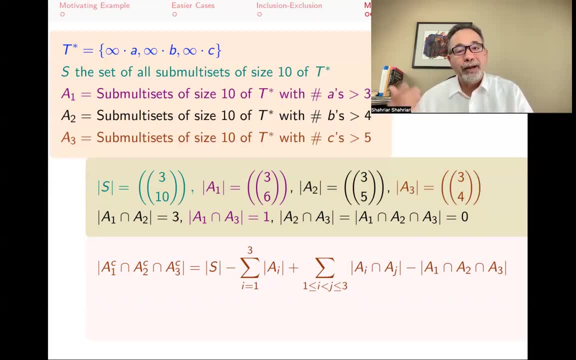 you subtract all the bad guys from a1, all the bad guys from a2, all the bad guys from a3, but you have overdone it. So you add in all the intersections of pairs of those subsets, but you have overdone it again. So you take out the intersection of three of them, Except in this. 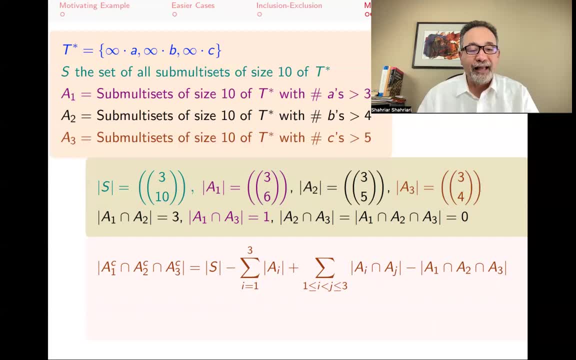 case. the last one is zero. You actually haven't overdone it in that last case. So if you put these numbers in, you will get this alternating sum. So the first one is the size of s. Then you have to subtract the three sizes of a's And then you add the three intersections of two of them And 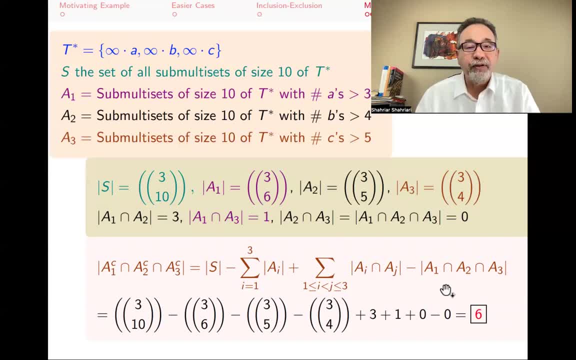 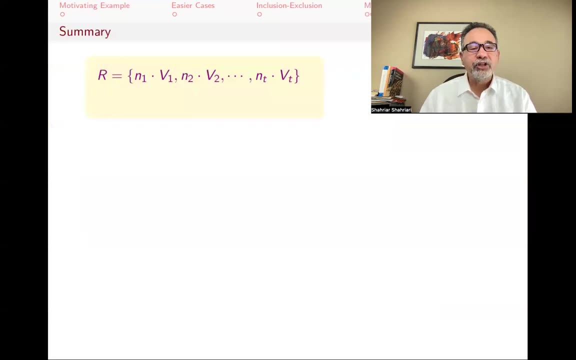 you subtract the last one And you get six, And actually the answer is small enough. Then it might have been easier to just actually write down what all the possibilities are, But this was a proof of concept, As they say in Persian. Okay, So what's the summary? The summary is that if you have 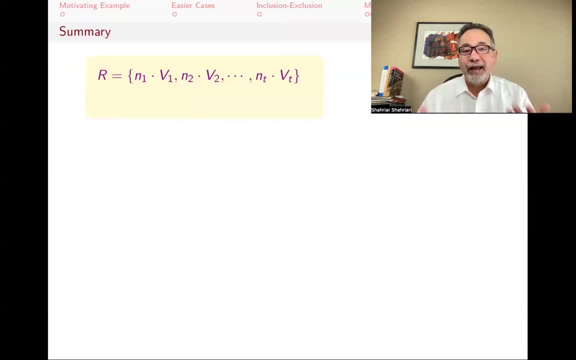 a multi-set with repetition, random repetition numbers n1,, n2, true nt And if you also have, if you want to deal with that, you want to find sub-multi-sets of that. you usually look at an accompanying multi-set that has less restrictions. Its restrictions are: 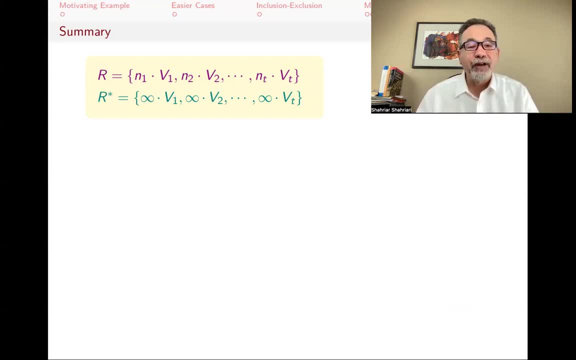 there is no restriction. There's infinite number of each one of the types of elements on that set because it's a multi-set. So if you have a multi-set that has less restrictions, there's no restriction. There's infinite number of each one of the types of elements on that set. 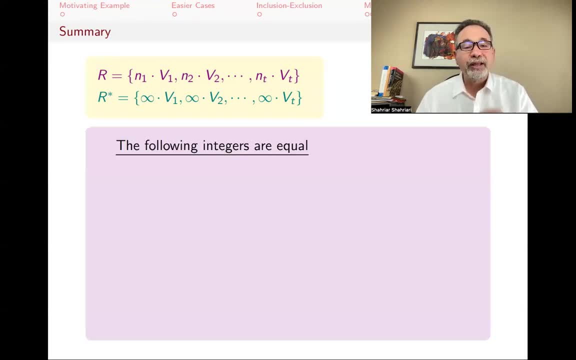 we call that r-star, Then what we just showed is that the following integers are equal: If you do any one of these things, you get the same answer. So one of them is that if you want to find the number of s combinations of r, So s is some number And you want to find, you want to choose s elements. 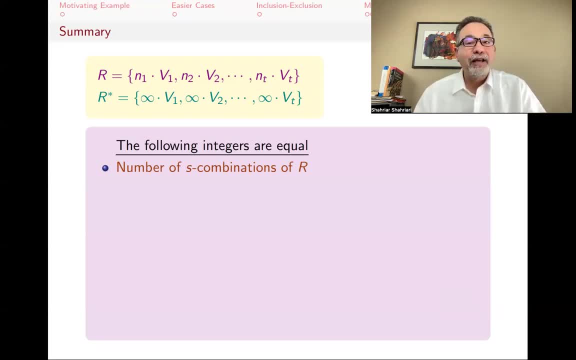 of r, But given the restrictions that r has, that it doesn't have, you can't, you might not be able to take all of the elements to be v1, because there might not be enough v1. There might be, but there might not be. So what am I saying about that? I'm saying that's the same as. 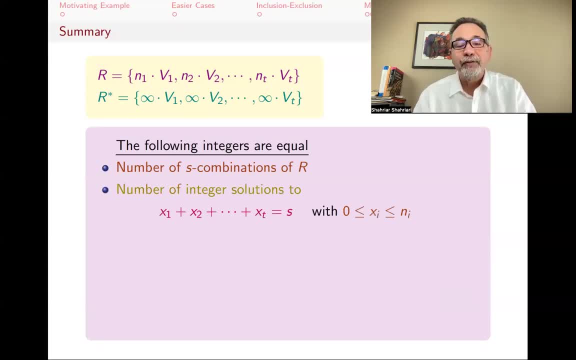 the number of integer solutions to x1 plus x2 plus xt equals s, which, each one of the xy having a restriction, x1 is between 0 and n1,, x2 is between 0 and n2, and all the way till xt is.